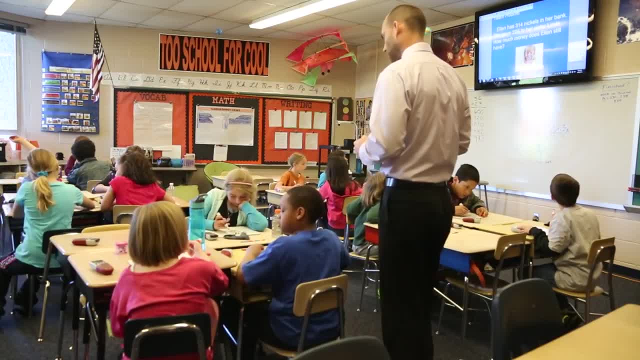 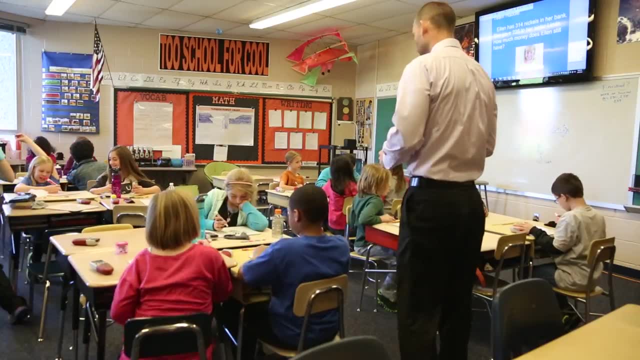 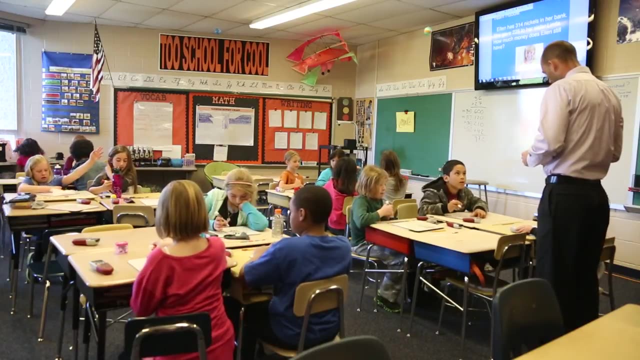 I thought it was nine minus two, I thought it was nine minus two, And then it was fourteen minus five. Okay, So she doesn't have a dollar, Not even a dollar left, so it's just eighty-nine cents. Now hold on. 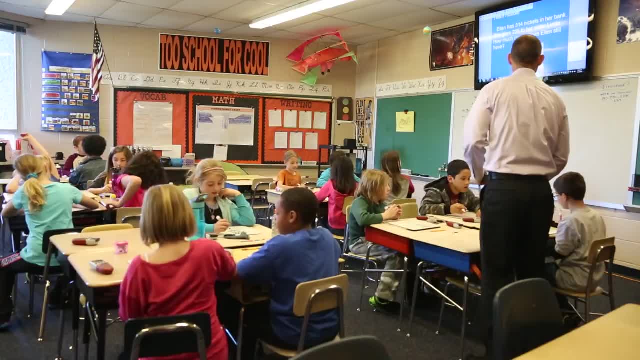 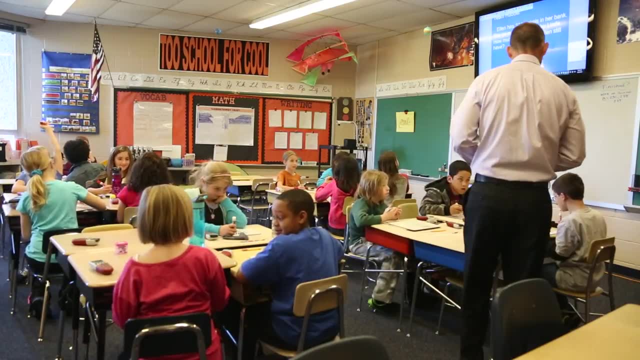 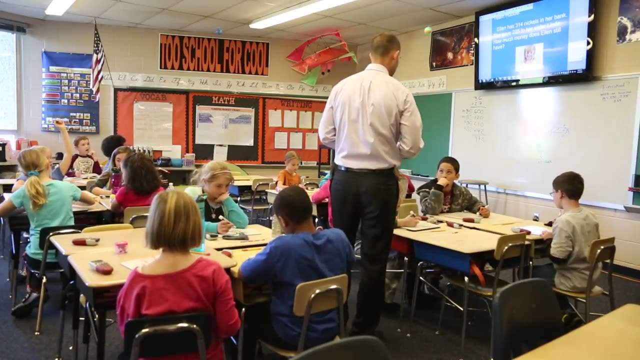 Are these pennies here? What are we talking about? You have eighty-nine. what Nickels, Nickels. So how much money is that? No money, One step, One step. Yeah, Let's find how much. We'll keep an eye on you. 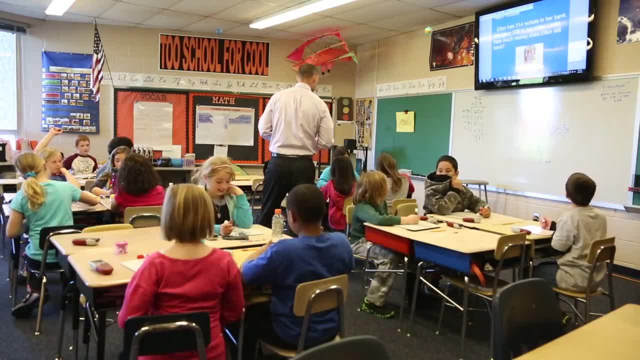 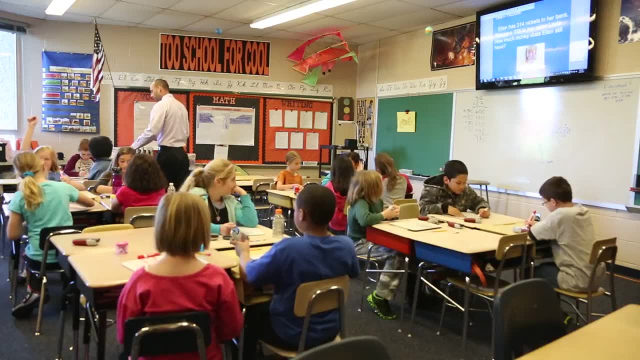 Eighty-nine cents. How about three? How about three hundred twenty? You all right, Mr Alex? Yeah, Keep that marker in your hand. So are you guys done yet? No, we were just trying to find out if it was division or subtraction. 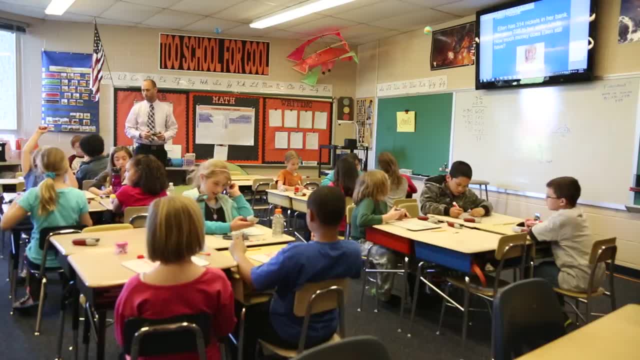 Okay, All right, So you started with a good first step. Okay, So what is this telling you? Eighty-nine what She got? eighty, She got eighty-nine nickels, All right. So what are you going to have to do to figure out how much money that is? 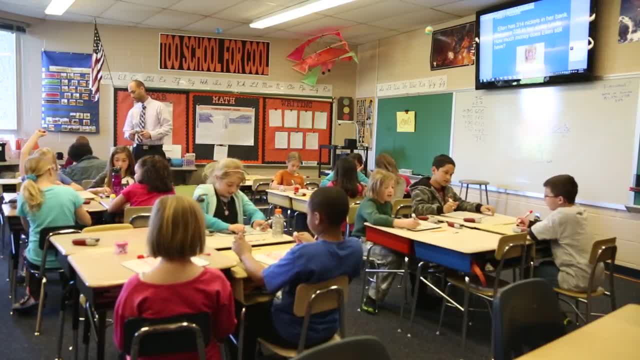 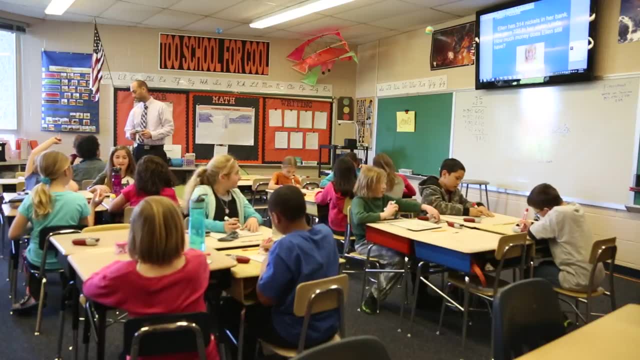 Two, Two. I said two, I was going to say two. Oh, Oh yeah, Maya. Oh my goodness, They're dropping like flies. Go get a new one. Two, Two, Two, Two, Two Two. 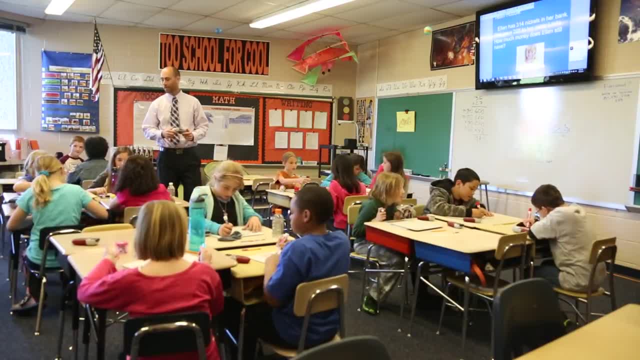 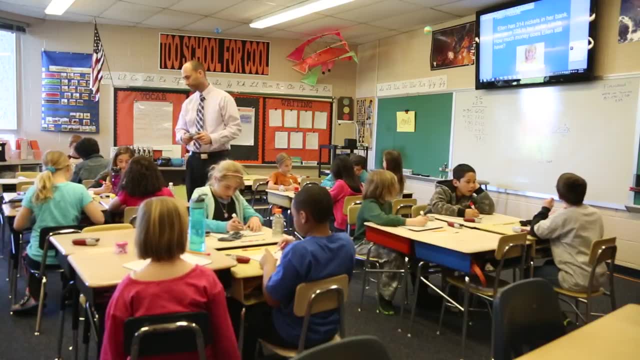 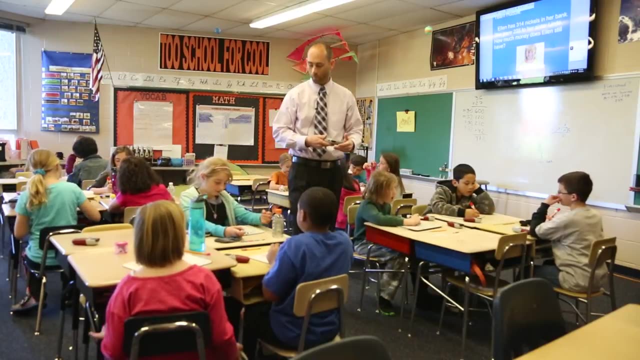 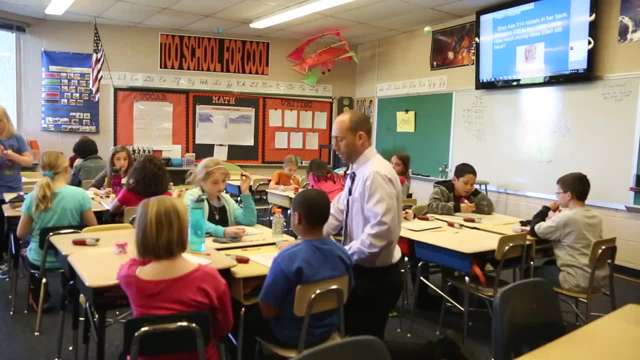 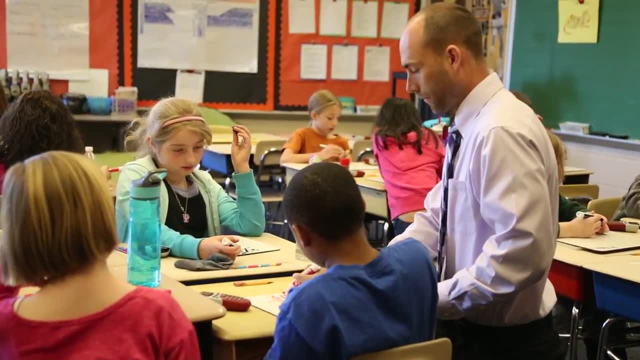 Yes, All right, We have a mistake. It's our mistake. Yes, We have to start over. Is four bigger than five? No, All right. So what do you need to do? Cross the one out and the Yup. 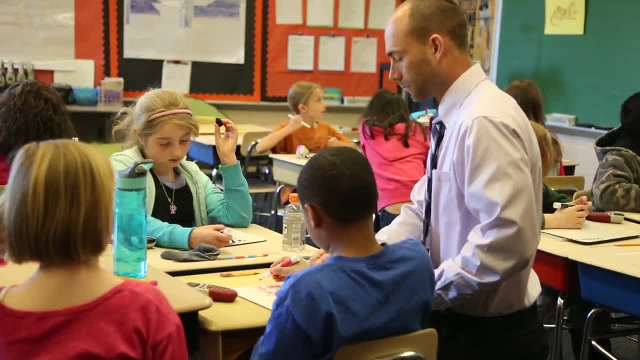 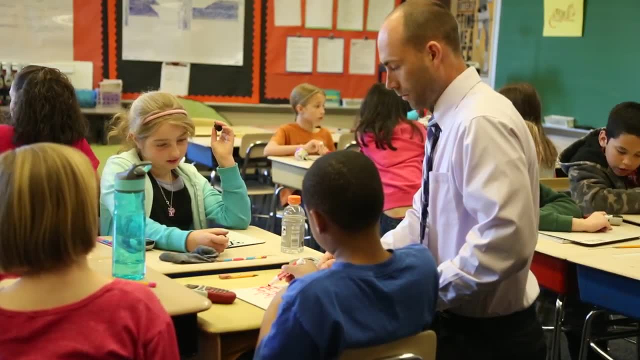 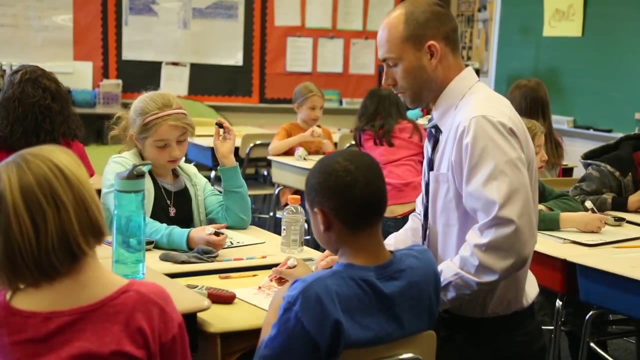 Fourteen, what happens to the one? all right now. zero bigger than two, all right. so what do we need to do? can't make it a 10 yet, unless we borrow where we're gonna borrow from, all right. so let's go ahead and do that. your three turns into a all. 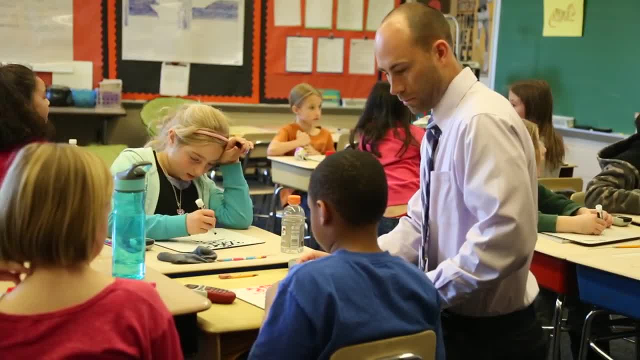 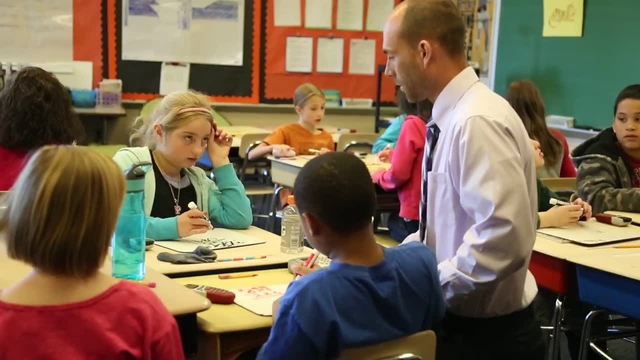 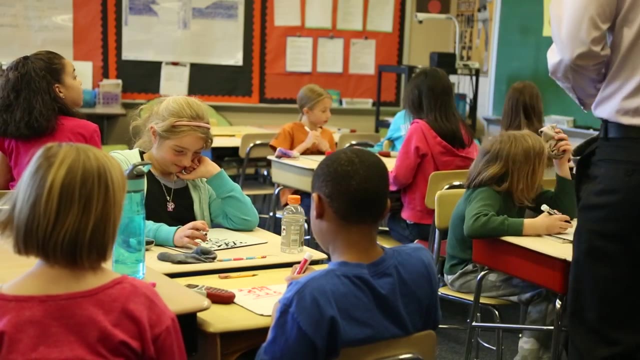 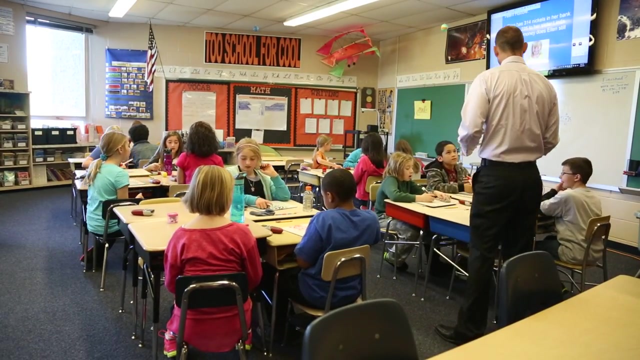 right, it's two greater than or equal to two. what's we do? it's equal to right. okay, so now go ahead and do your subtraction. okay, 89 nickels. you figured out how many nickels. how are you gonna figure out how much money that's worth? how much is a nickel worth this way? five, what so you? 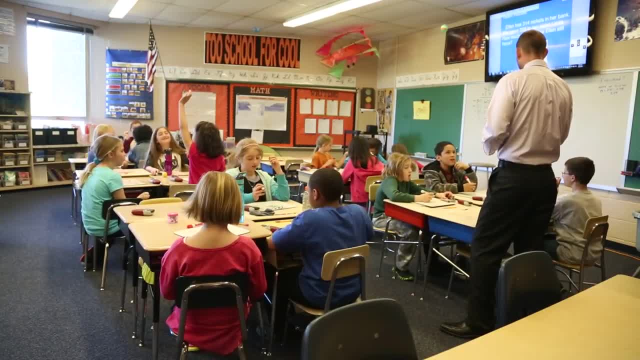 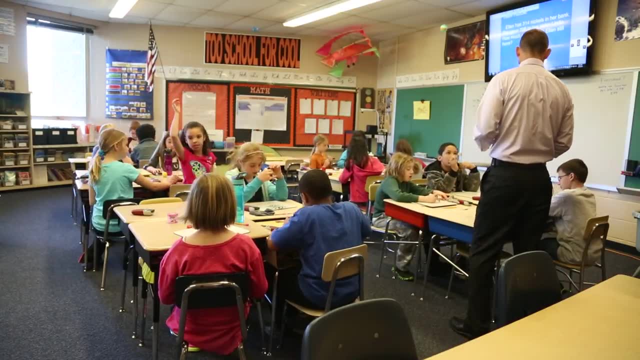 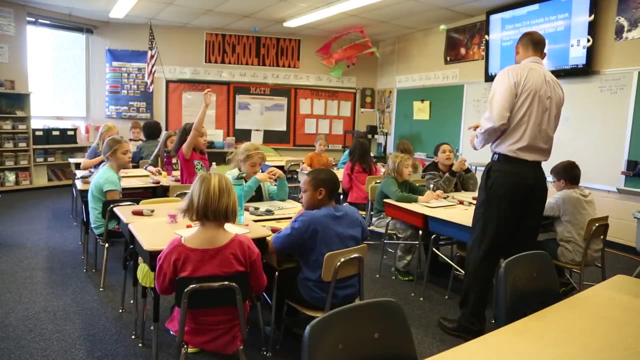 have 89 nickels. every single one of those nickels is worth five cents. so what are you gonna have to do? if I do 89 minus five, is that gonna tell me how much money I have every nickels worth five cents? I've got 89 nickels you got. 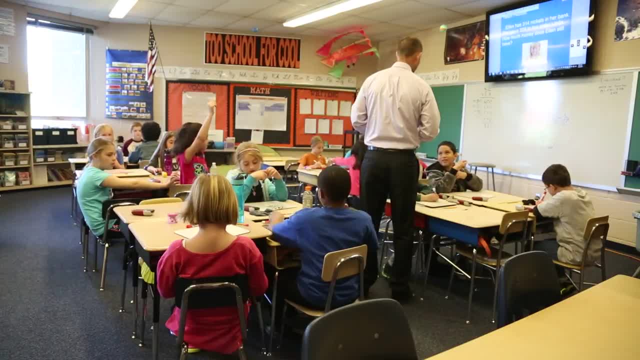 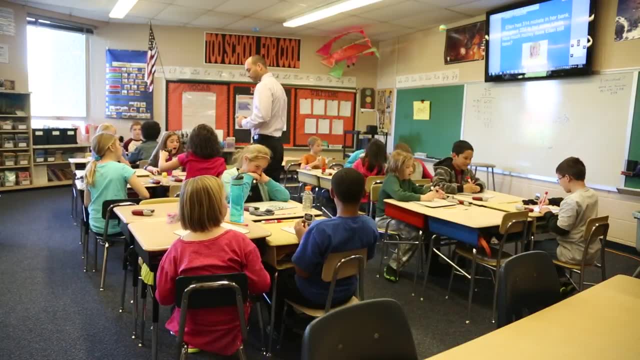 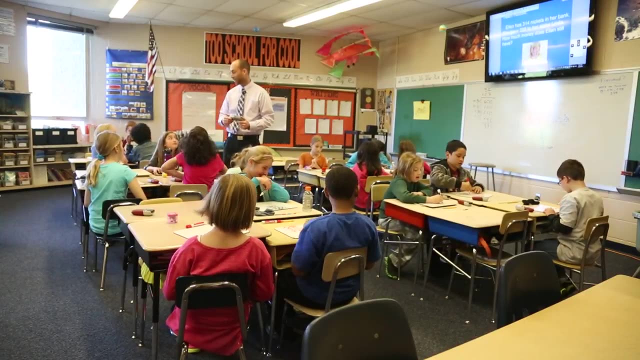 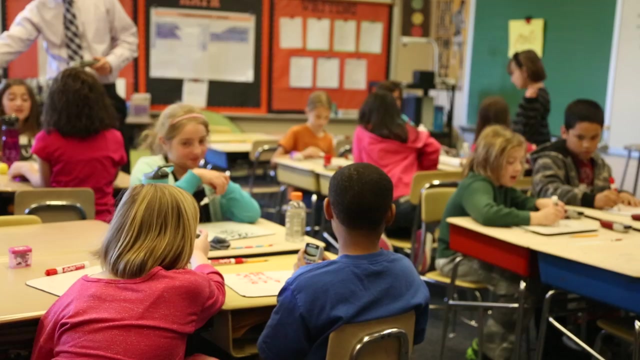 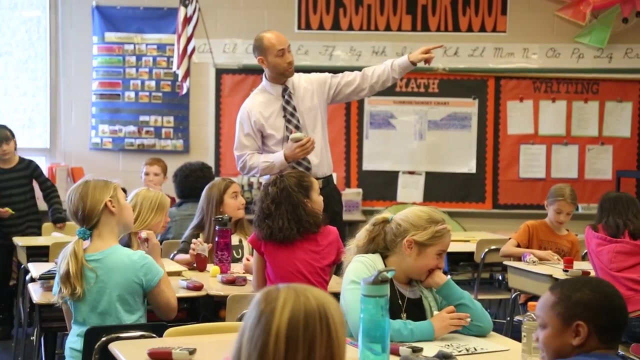 it. oh, you knew I was gonna call on you. Oh, jump to the gun a little bit. you've got to remember. your final step is: does my answer answer the question? is that saying I have 89 cents? well, let's figure it out. you subtracted 314 and 225, right? what are each of those things? 314, what? 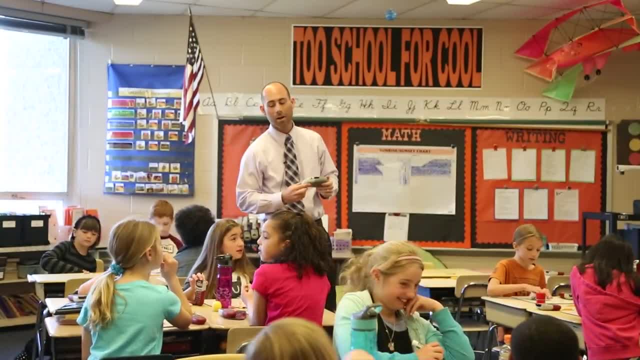 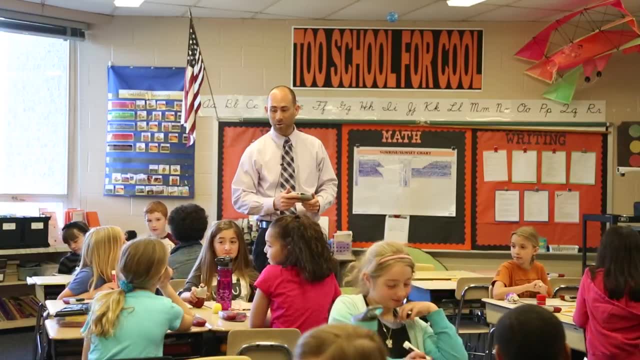 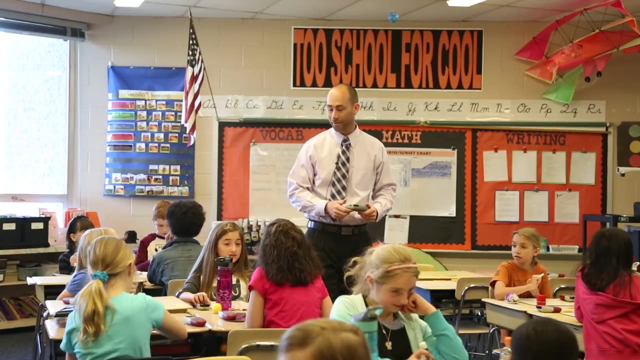 am I talking about cents or nickels? all right, you subtracted them. you have 89 nickels left over. how much money is that? how much is a nickel worth five cents? I've got 89 of them. how am I gonna figure out how much money that is? you got it? welcome back, miss Aubrey. oh, what am I? 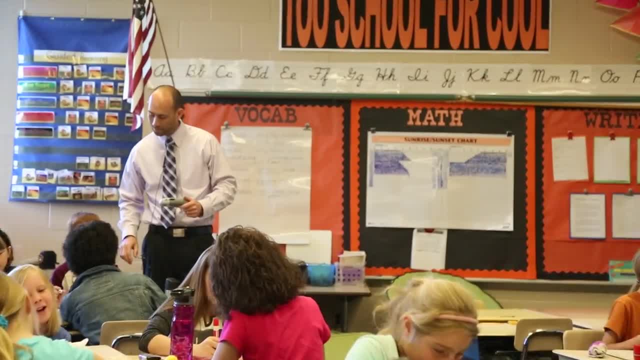 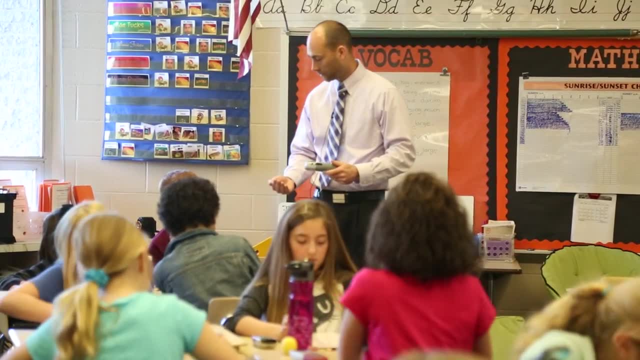 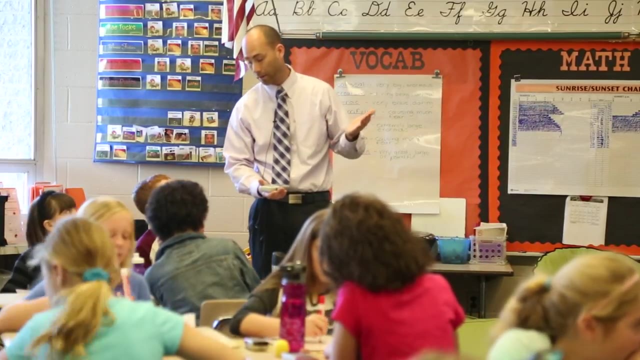 doing here? no, no, what are we doing? all right, you guys subtracted 314 and 225, right, and that gave you 89. you have 314 nickels and 225 nickels. we're through a. 225 of those nickels were given away. ship 89 nickels left over, so you guys got. 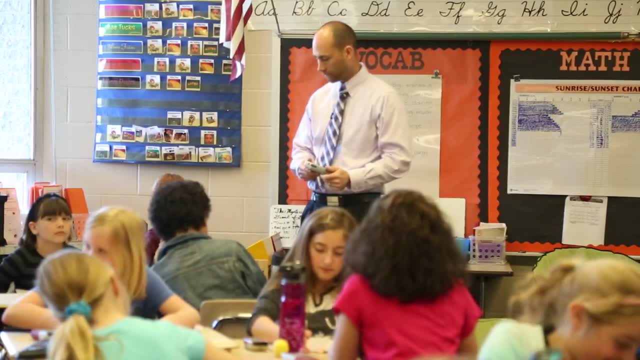 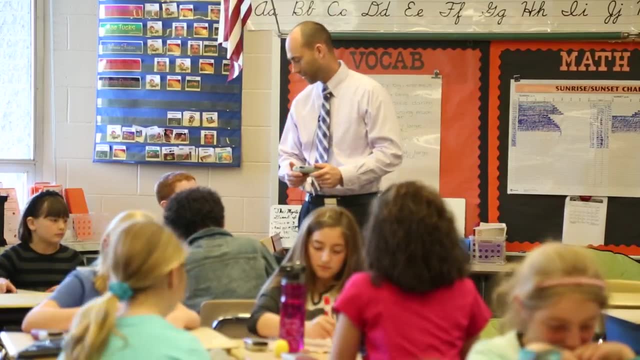 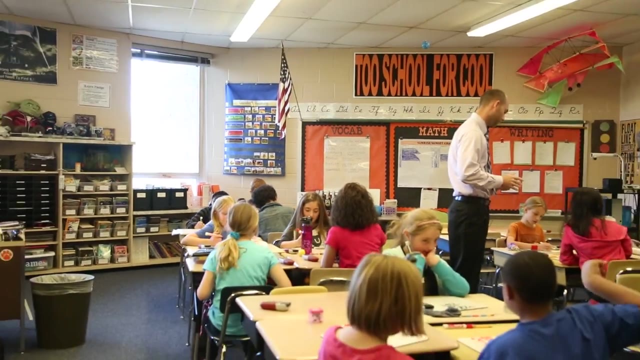 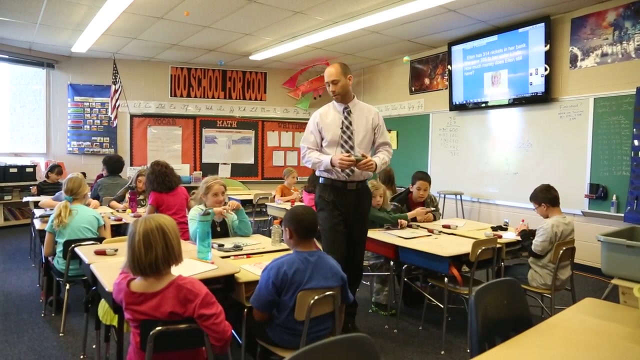 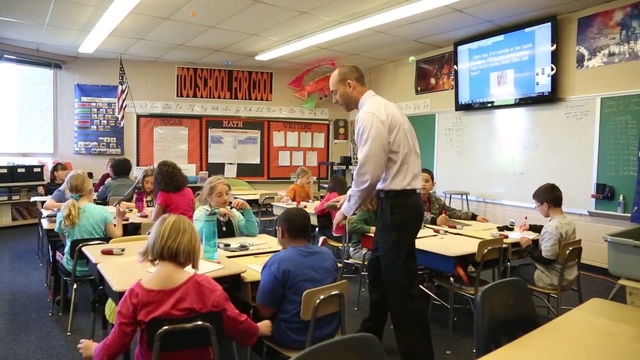 that step done. how much is a nickel worth five cents? you have 89 nickels. how much money is that? cha-ching, cha-ching, Oh, Oh well, are you done? yet we got it the same way. oh ho ho, all right, you guys got halfway there. 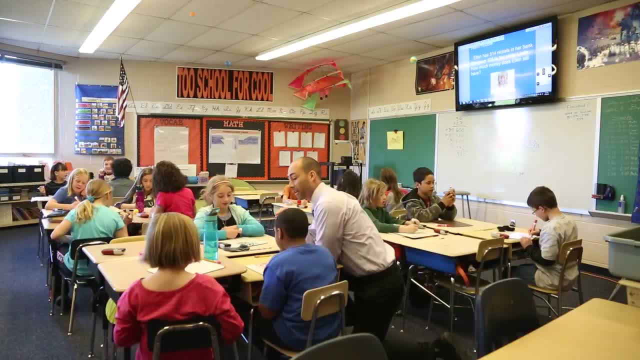 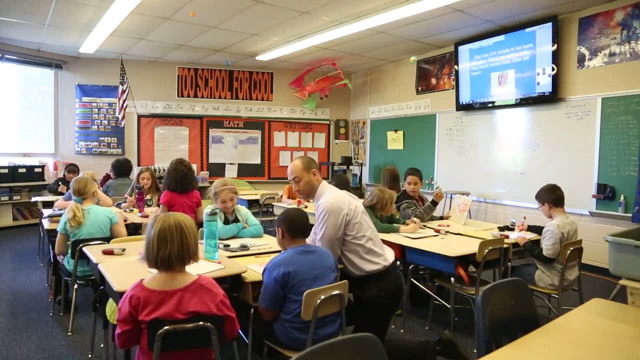 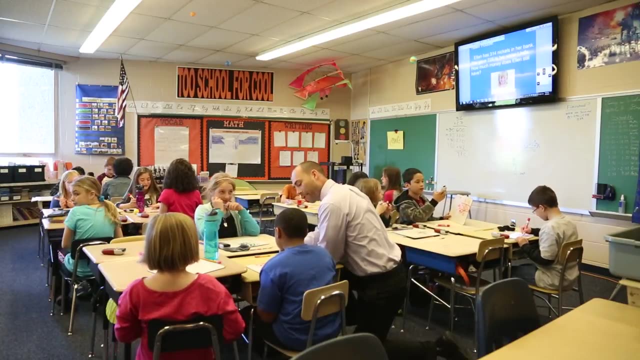 I said: we got it done. you got halfway there, right. so you had 314 nickels. Ellen did. she gave 225 of them to Linda. how many nickels are left over? but the question is: how much money does Ellen still have? does she have 89 cents or 89 nickels? 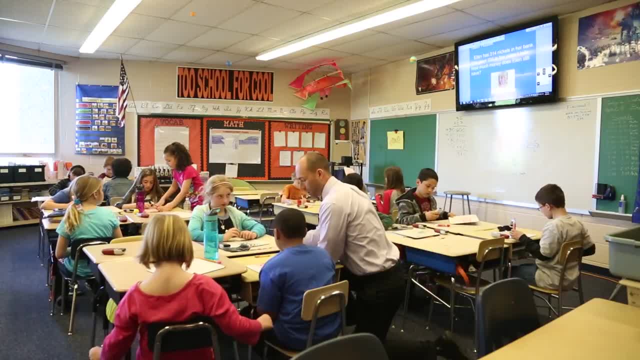 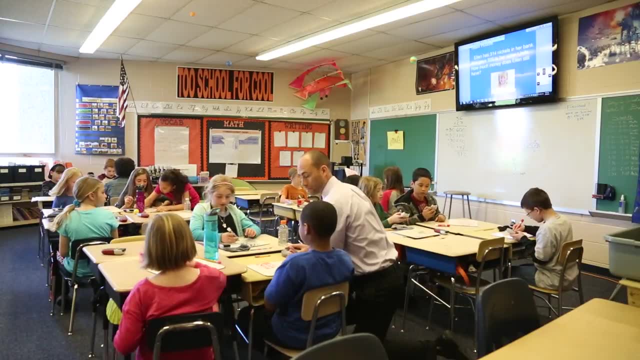 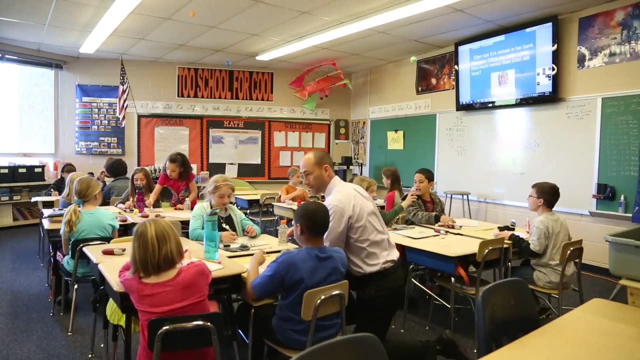 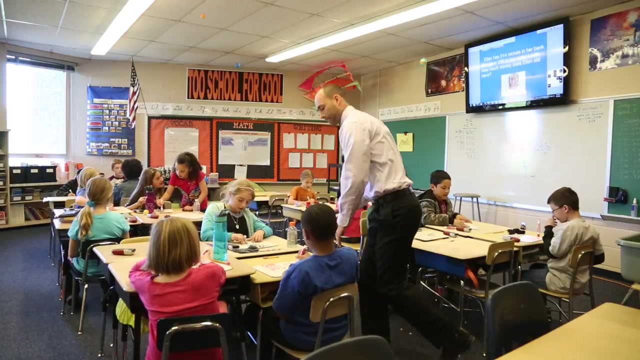 89. all right, how much is 89 nickels? you might not have it right on here, but you can get it right on your whiteboard, all right. so if you, I want you to try this out. each nickels worth how much? five cents, anyway, works for me. 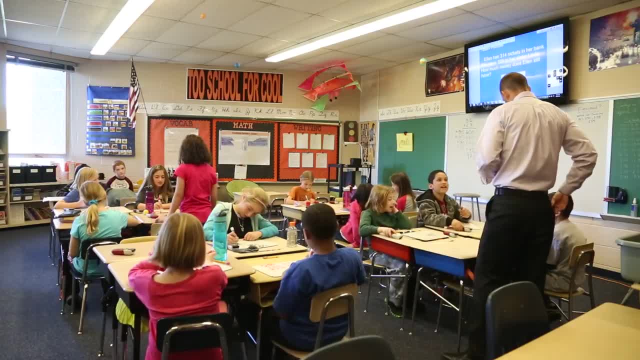 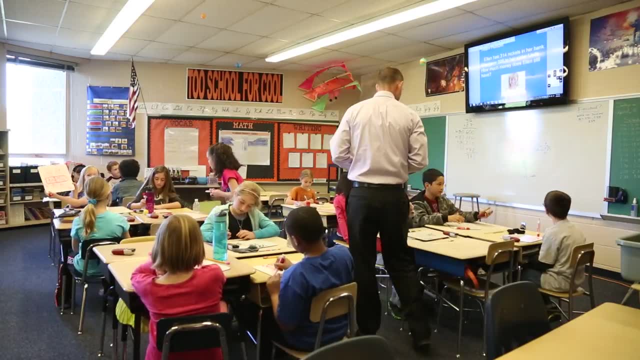 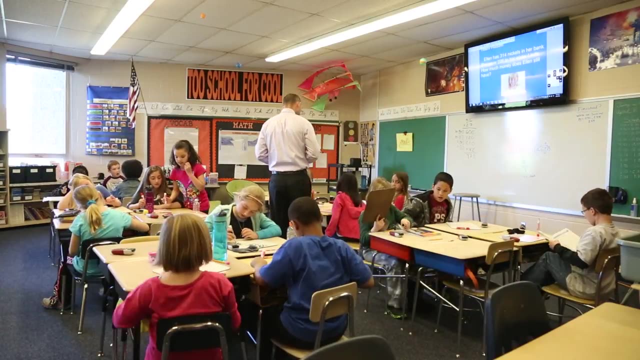 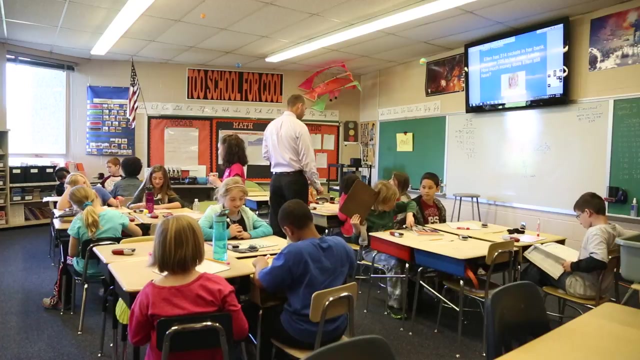 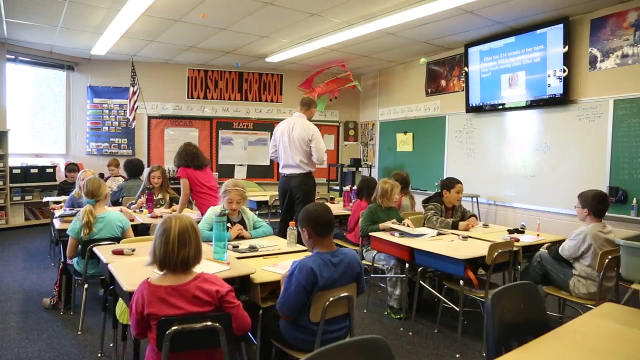 yeah, all right, you guys got it nicely done. good, good journal pages. whose is this? that's right, you're not sitting there. okay, what was the first thing you guys did? looks like you did 314 minus 225. what does that give you 91 cents. okay, I'm gonna tell you you guys did everything right. you're gonna subtract. 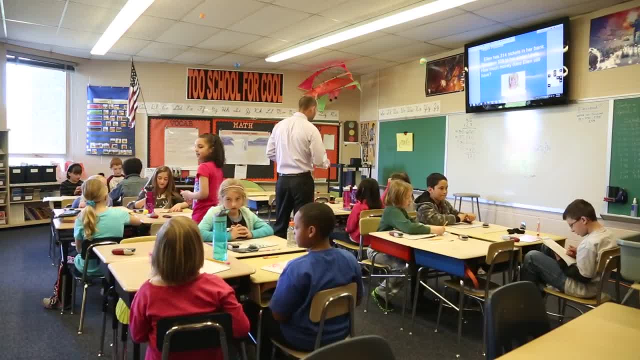 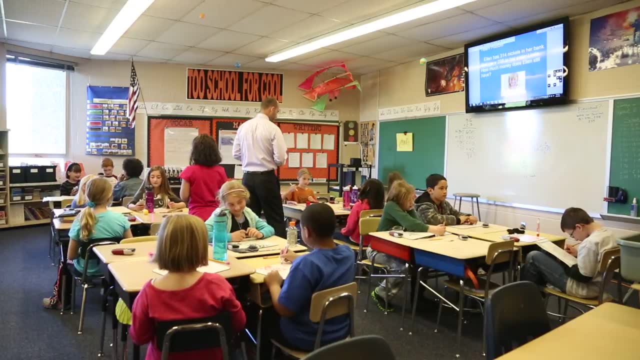 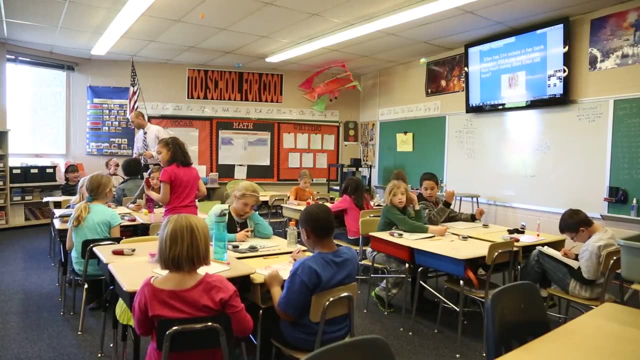 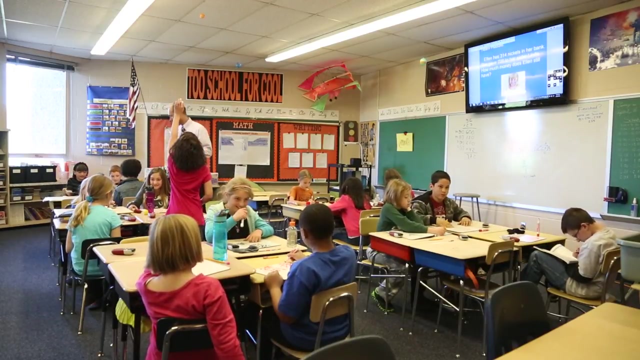 and then multiply. you did that, but your subtraction- you made an error on 314 minus 225 is not 91. check that out, are you guys done? yeah, did you get it right? nicely done. get on your math math boxes- good, good math boxes. don't erase it. don't erase it. leave it on there. I want to see the work. 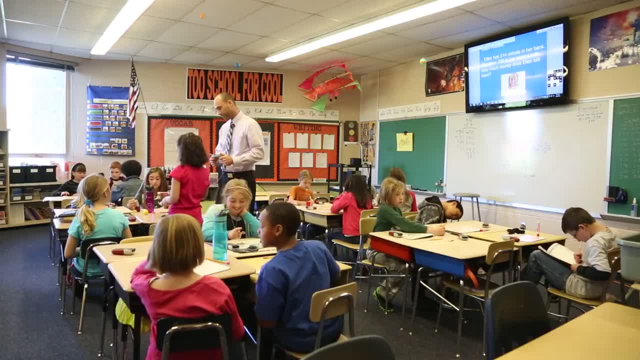 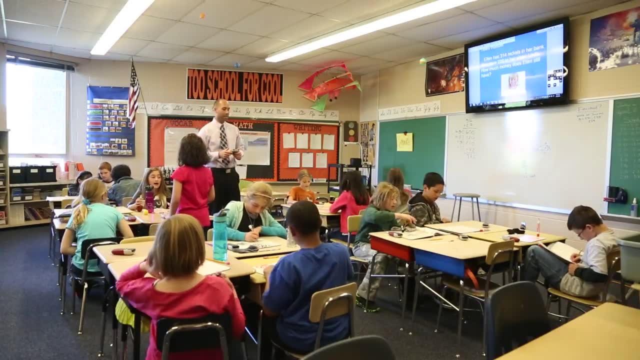 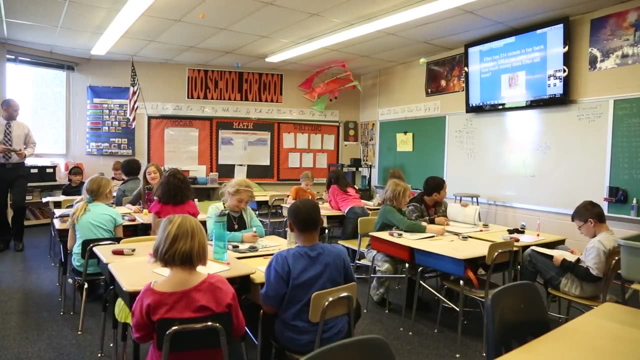 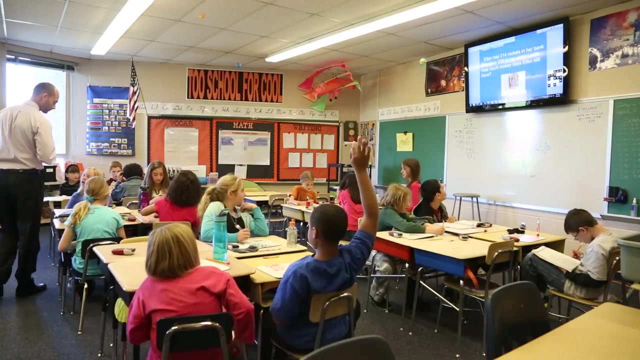 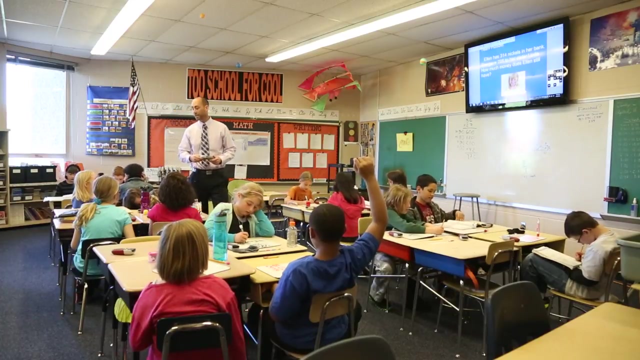 yes, I guess a little early. you have about one minute to finish this up. if you're not quite finished yet, alright, if you guys are done, go ahead and your math boxes. you can just leave that journal out. Maya and Maya. you understand, though. right, you guys did get the right answer. 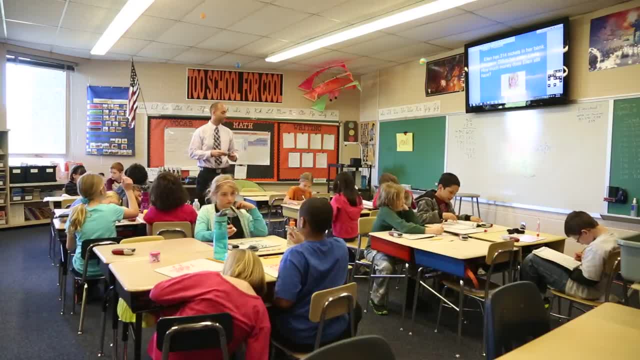 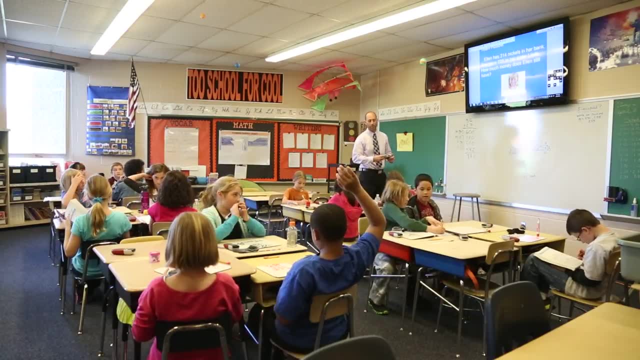 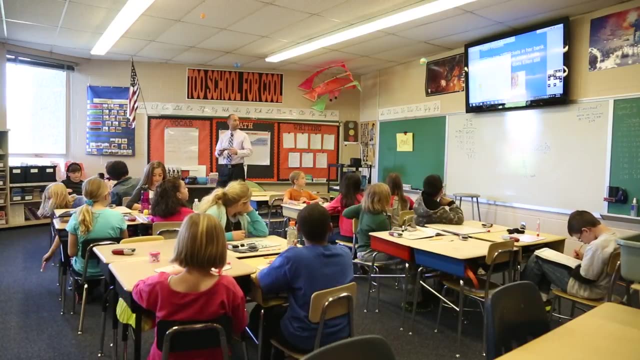 just not on your SRS. clap once if you can hear me, clap twice. if you can hear me clap three times, you can hear me tap your markers, fold your hands and look up here, if you can hear me. all right, let's take a look. eight of us said 445, five of us said 89 and of that, 485 of us said 445.. 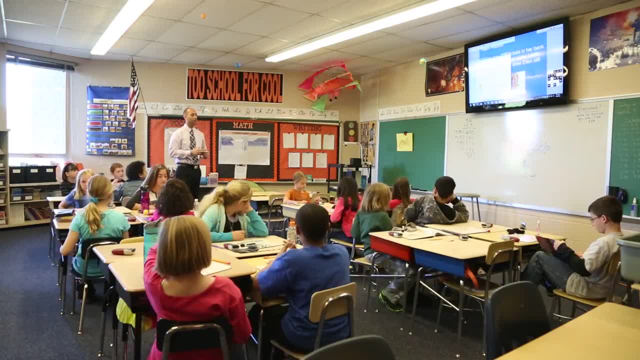 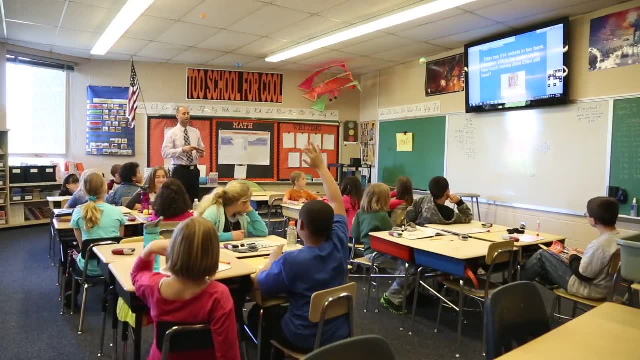 Okay, I got it. I got it. I got it. five I know of about four that ended up fixing it and getting the answer. So pretty good job all together. Do I have a volunteer? I'll take a volunteer, because these are difficult questions- A volunteer to go up there be the teacher, just like Lily was. Take my job. 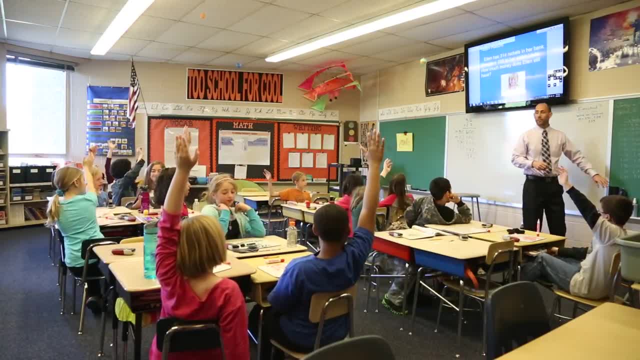 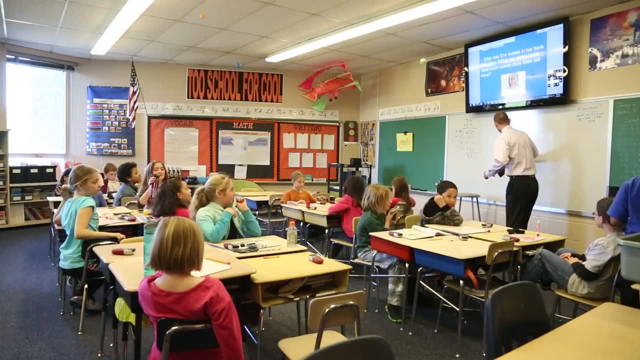 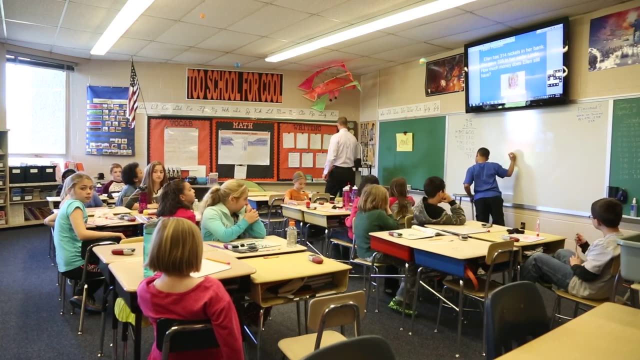 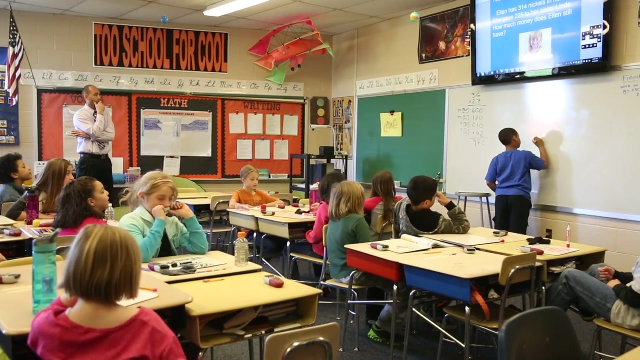 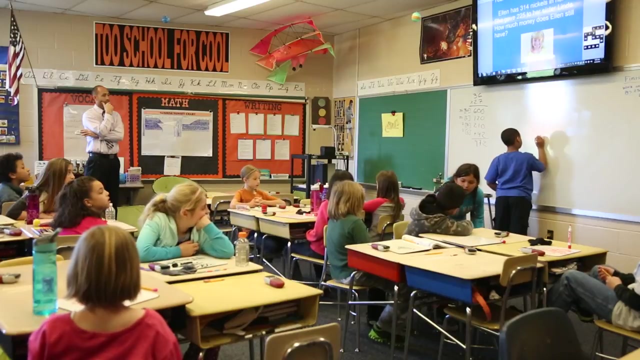 I'm still going to keep my paycheck, but you get to do my job for me. A volunteer- Mr Jameer- has been on the ball today, So I'll let Mr Jameer come on up here Tell us how you did it. So first I did 314 and 221. Then I knew that you couldn't put that away you. 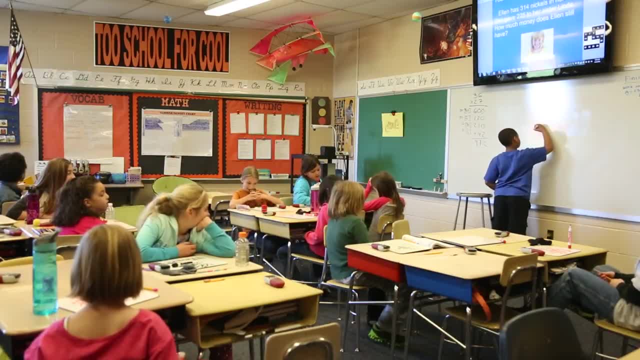 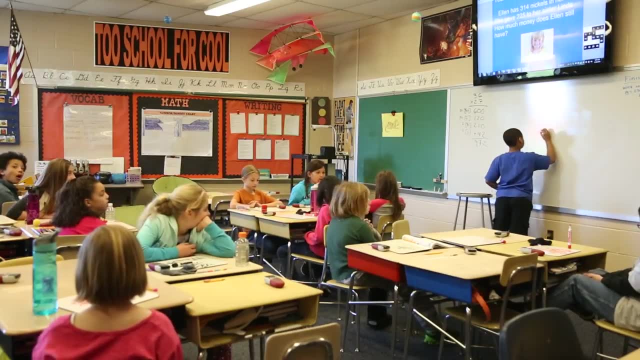 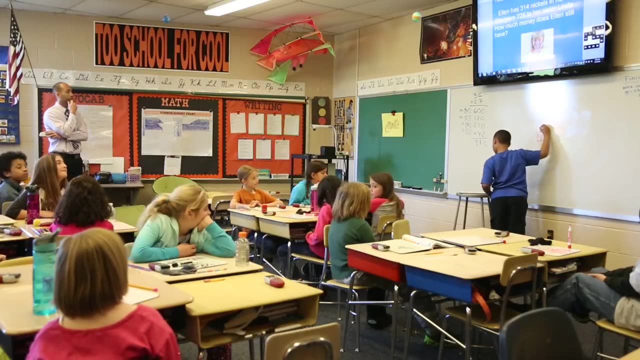 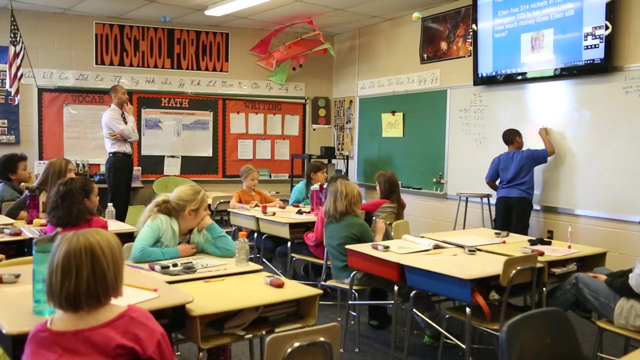 couldn't subtract one from two, so like one's not the same, Make that a two and make the one a ten. Then I knew it becomes subtract four from five. so I made it this A one ten. Good, you caught it. Thumbs up if you started off by subtracting. 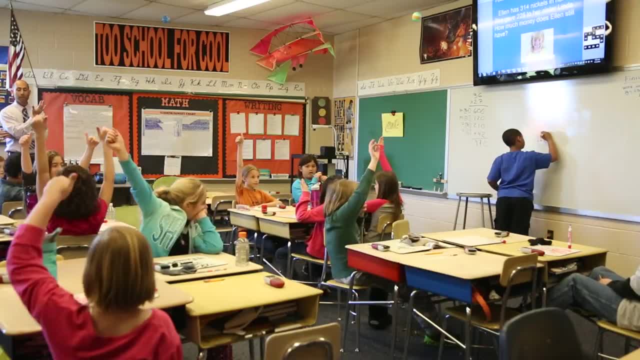 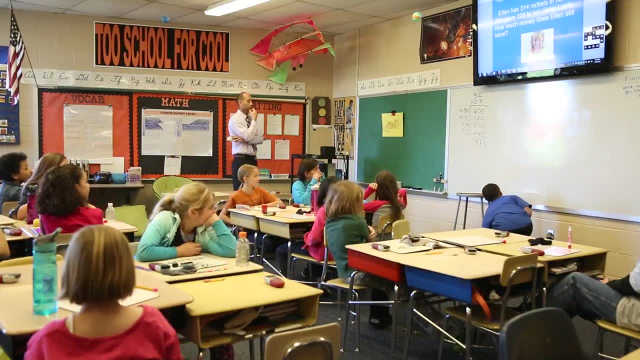 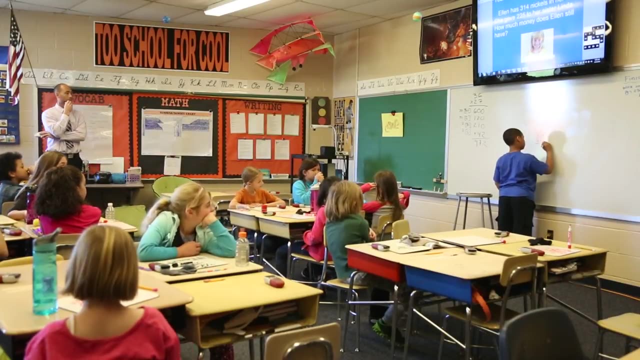 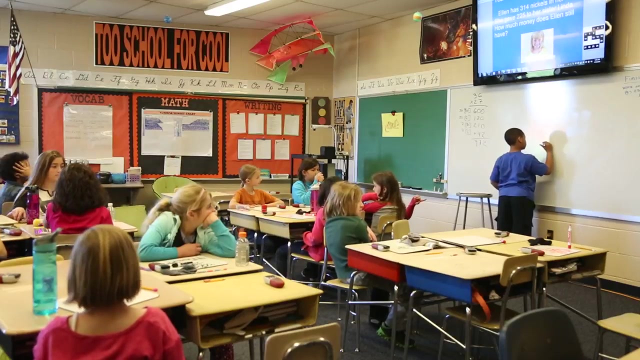 314 and 225.. Good, first step. Now you're going to figure out how many nickels she has left over. Matthew, would you shut the door? Thank you, Put it away, or I take it. Fourteen from five is nine. Ten from two is two. 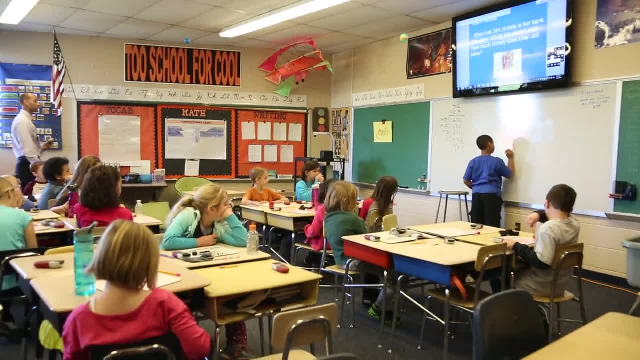 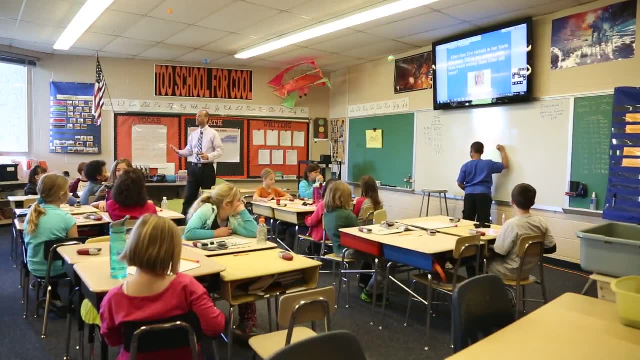 Okay, Two from two is zero. I knew I wasn't finished so I had to do it. I had a couple of you stop at 89. It felt like you were done, But remember, these are 89. what Aniyah? 89?. 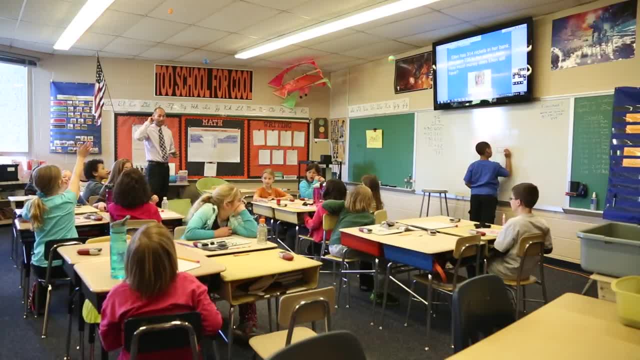 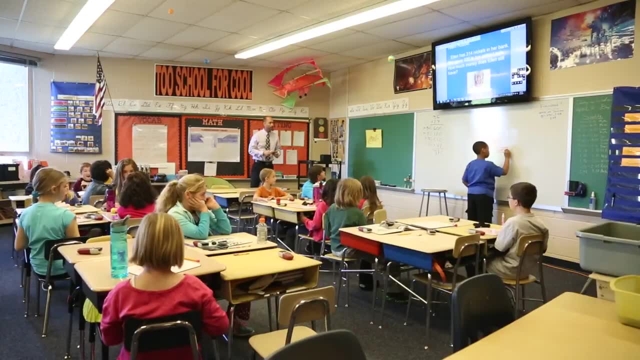 Cents, Not 89 cents, 89 nickels. So we've got to figure out if I have 89 nickels, how much money do I have? And I have a lot of my students loving the lattice method today- A lot. I don't. 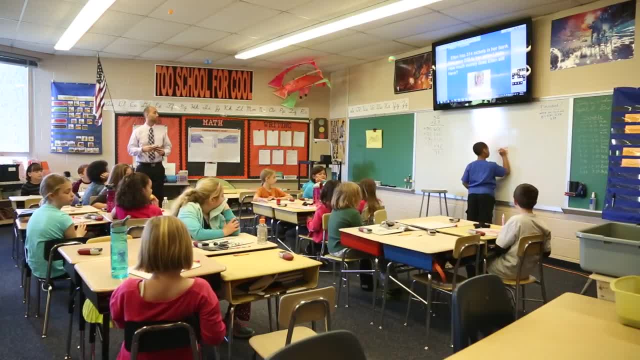 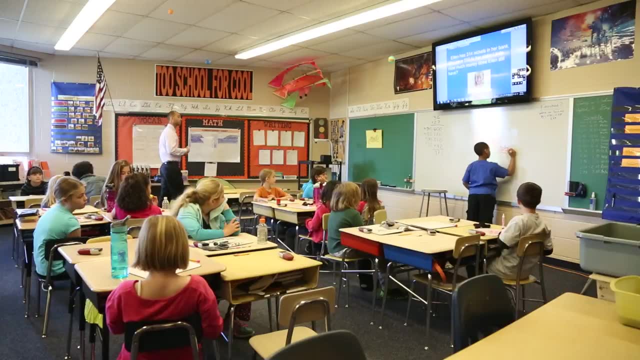 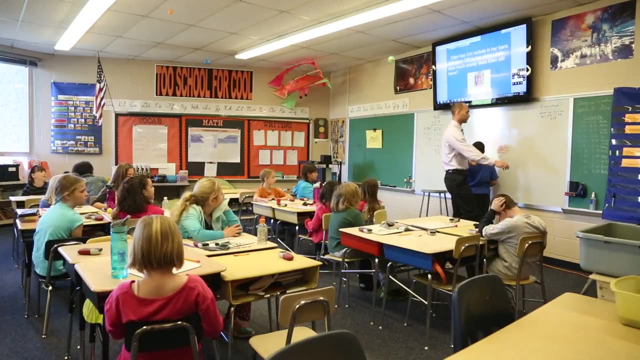 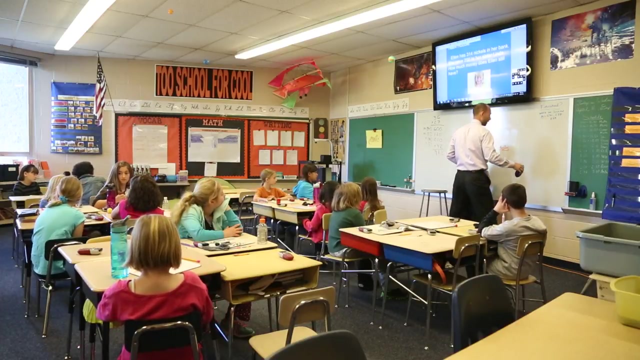 I do, I do, I do 89.. I did five times. Let me help you out here, Jameer: Remember this is single digits, so you only need one. And five times eight is not ten, Five times eight is 30.. 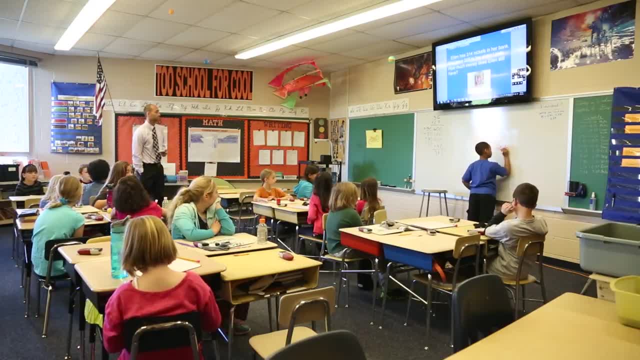 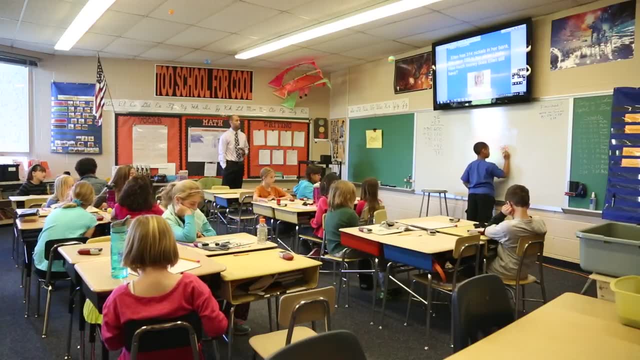 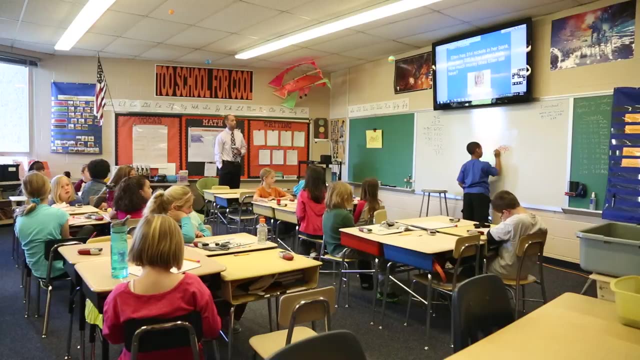 Nine Nine times five is 45. And I did. I had a three-count subtraction: Zero from five is a five, One from zero is a four, And four from three is a four. Okay, so we have 445. what, Jameer? Nickels, Nope 445. what Cents? 445 cents. Is there another way we could say: 445 cents, Four dollars and 45 cents, Four dollars and 45 cents. Either way, you are correct, Jameer. what cheer do you want? 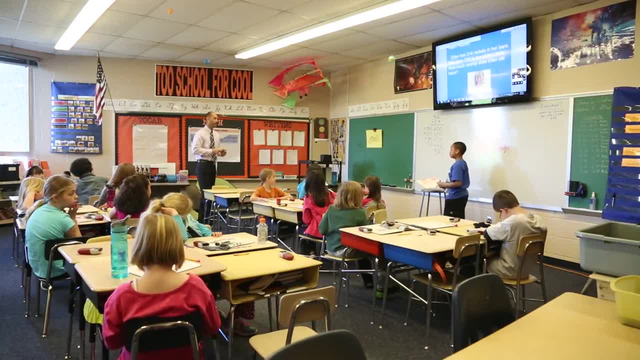 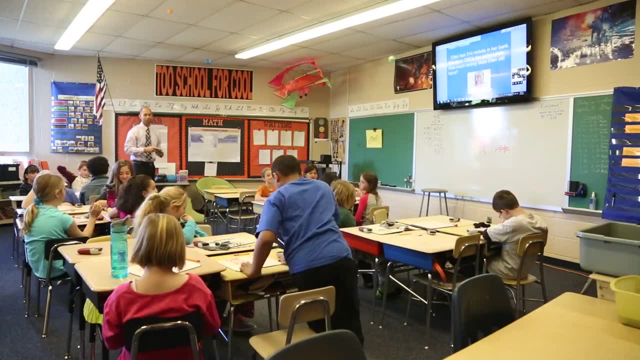 There's no mmm cheer The zombie, cheer The zombie, cheer Ready. It kind of sounded like what he said: All right, guys, are you ready for the next one? All right, hands on your eyes. I don't want you peeking.